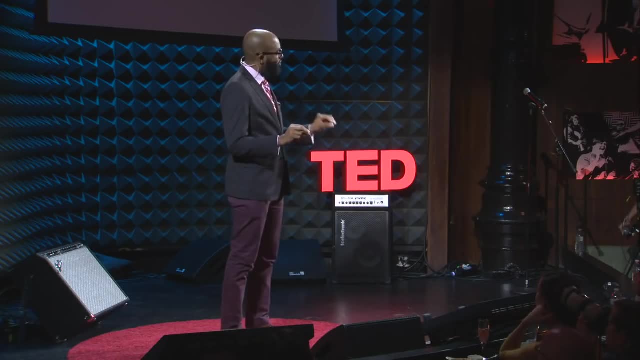 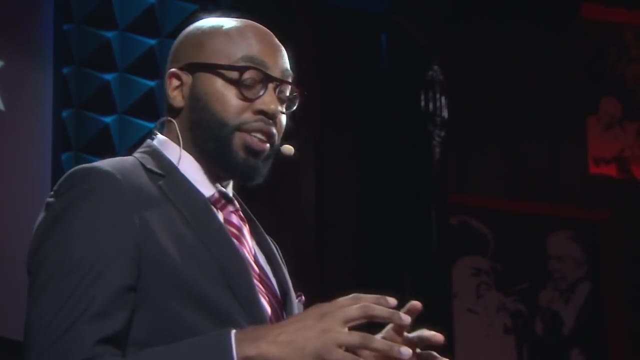 he's very, very sick and can't make it to school tomorrow. On the other hand, right now, there are amazing educators that are sharing information, information that's shared in such a beautiful way that the students are sitting at the edge of their 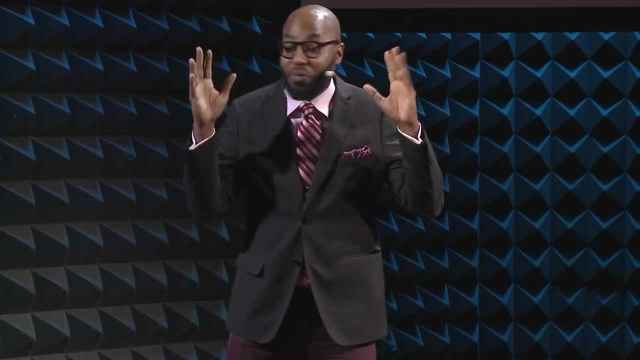 seats just waiting for a bead of sweat to drop off the ceiling. Right now, there is a student who is coming up with a way to convince his mom or dad that he's very, very sick and can't make it to school tomorrow. And right now that's меня, parent-in- law for the families whose daughter is carrying. 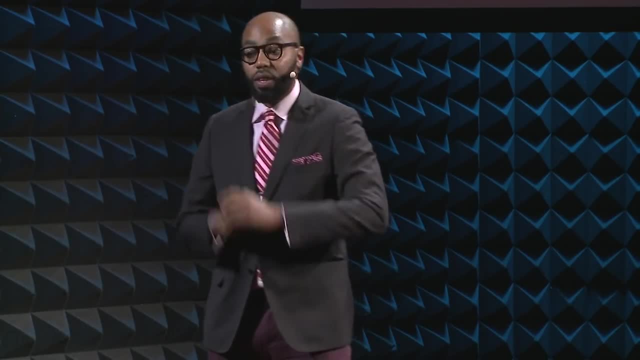 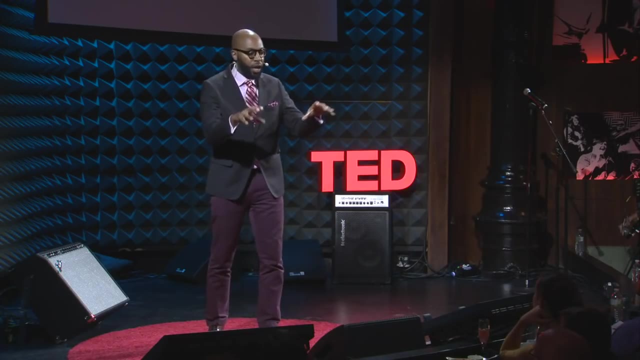 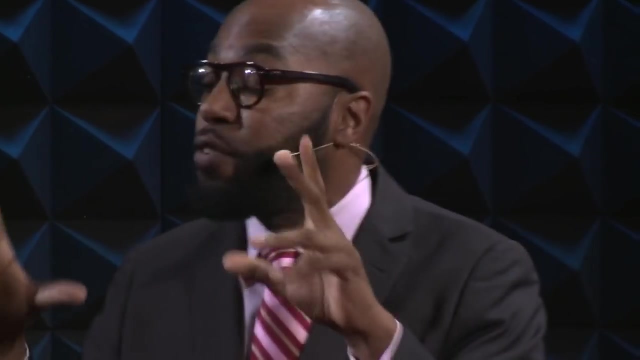 all of this information to Monroe County. Right now there is a third-year teacher at home who is saying: but my weight isn't even taxing— уровrize my commute fees. The reason for that is because the kid who's listening is not Denton's dad. 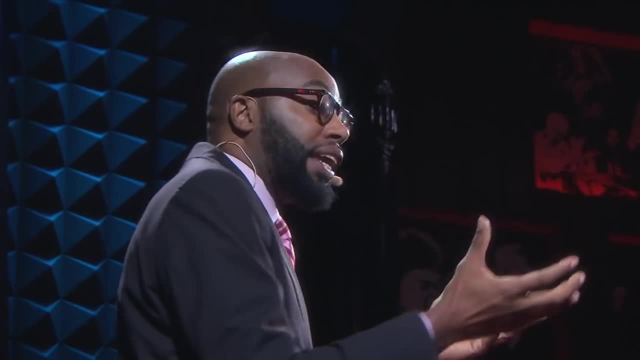 They're just engrossed in local history, And right now this teacher is expelling all that knowledge from his mom or dad on television. See Wahrad. as far as technology goes, all that information is exploring him or her— and they hire en unbelievable people. 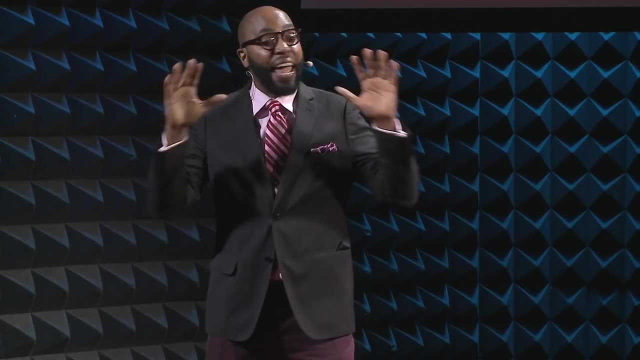 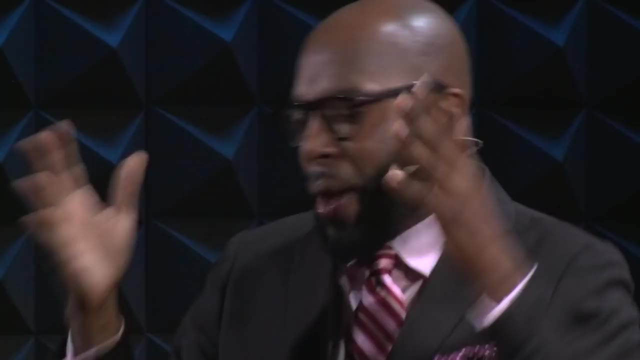 But right now— There's a person who can tell an audience to put their hands up in the air and they will stay there until he says: put them down right now. So people will then say: well, Chris, you describe the guy who's going through some awful training. 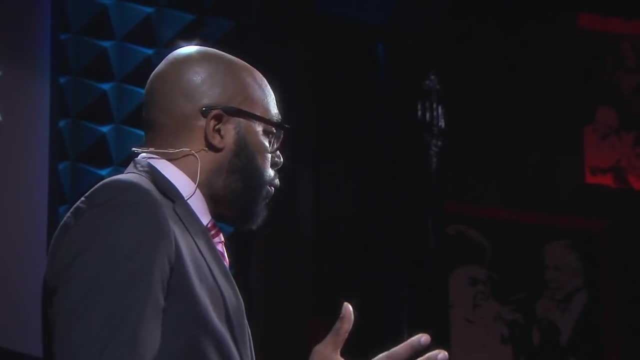 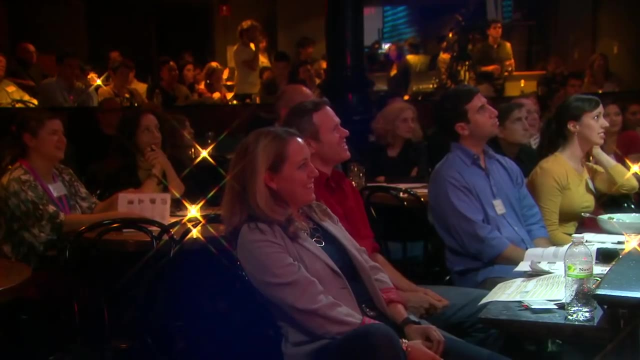 but you're also describing these powerful educators. If you're thinking about the world of education, or urban education in particular, these guys will probably cancel each other out and then we'll be okay. The reality is the folks I described as the master teachers. 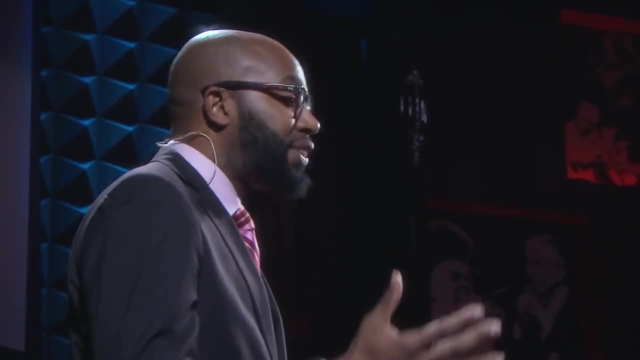 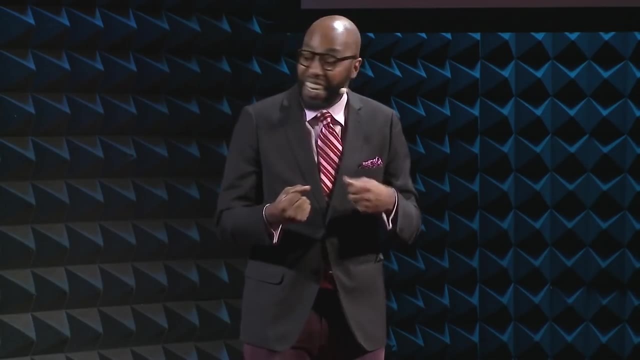 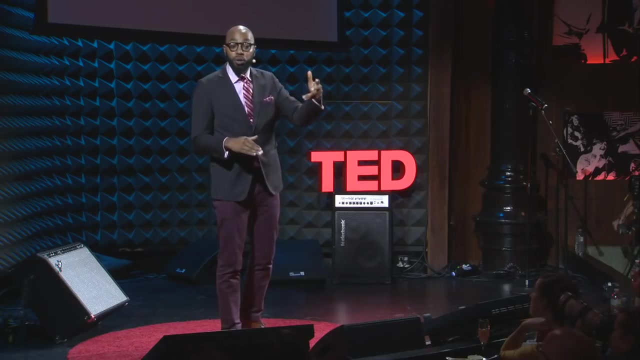 the master narrative builders, the master storytellers, are far removed from classrooms. The folks who know the skills about how to teach and engage an audience don't even know what teacher certification means. They may not even have the degrees to be able to have anything to call an education. 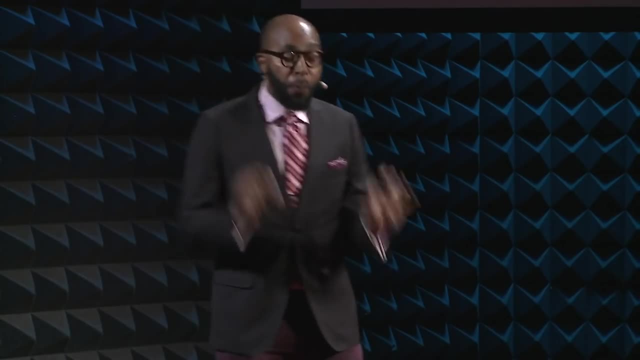 And that, to me, is sad. It's sad because the people who I described that were very disinterested in the learning process want to be the ones who are teaching, want to be the ones who are teaching. They want to be effective teachers. 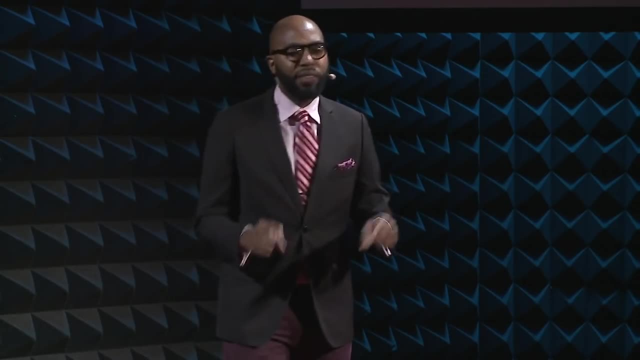 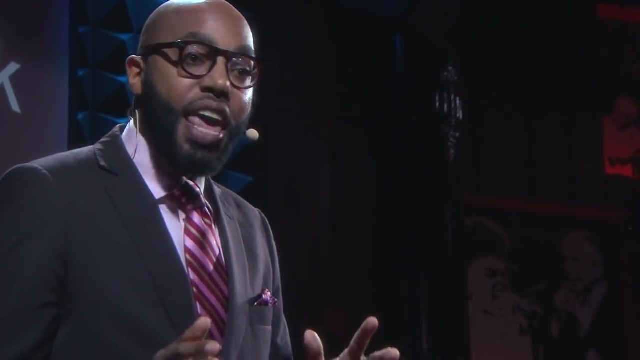 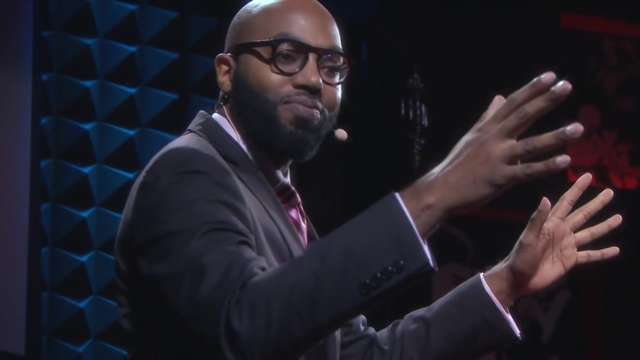 but they have no models. I'm going to paraphrase Mark Twain. Mark Twain says that proper preparation or teaching is so powerful that it can turn bad morals to good. It can turn awful practices into powerful ones. It can change men and transform them into angels. 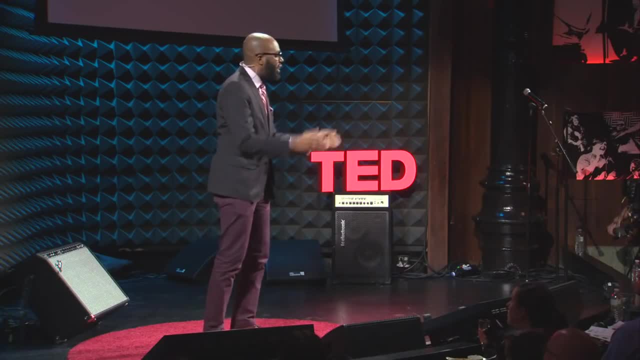 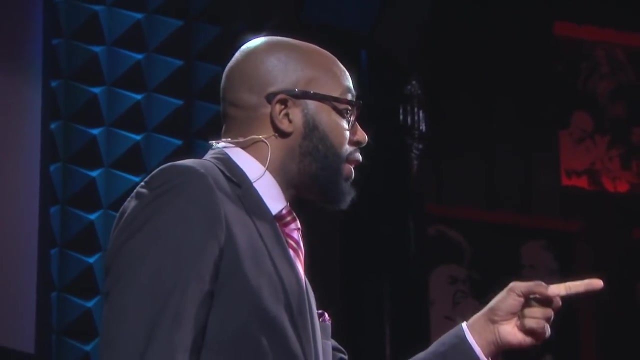 The folks who I described earlier got proper preparation and teaching, not in any college or university, but by virtue of just being in the same spaces as those who engage. Guess where those places are: Barbershops, rap concerts and, most importantly, in the black church. 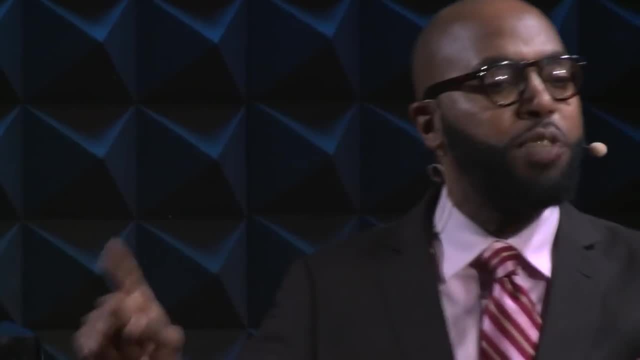 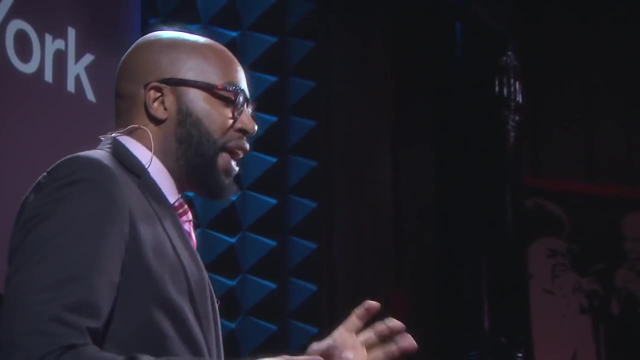 And I've been framing this idea called Pentecostal pedagogy. Who here has been to a black church? You got a couple of hands To go to a black church. that preacher starts off and he realizes that he has to engage the audience. 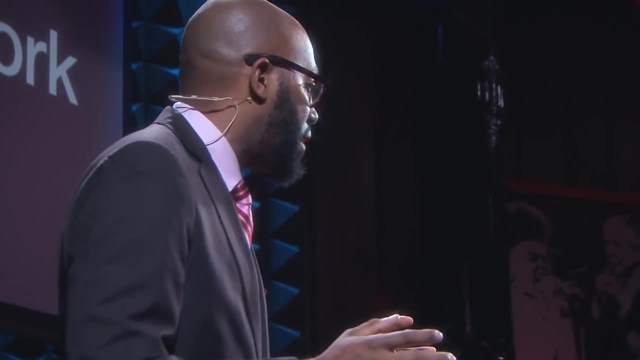 So he starts off with this sort of word play in the beginning oftentimes, And then he takes a pause and he says, oh my gosh, they're not quite paying attention. So he says, can I get an amen? Amen. 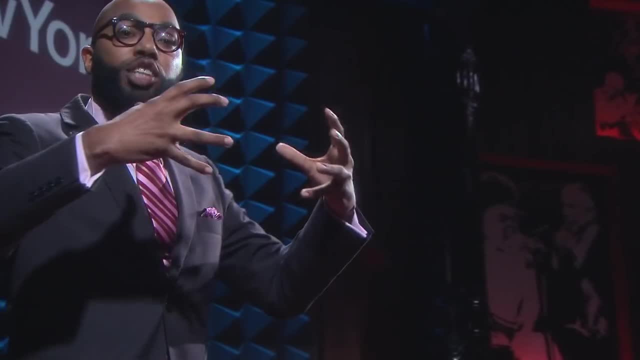 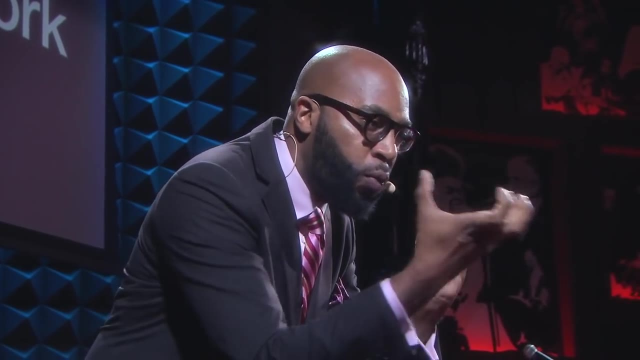 So can I get an amen, Amen. And all of a sudden everybody's reawoken. That preacher bangs on the pulpit for attention. He drops his voice at a very, very low volume when he wants people to key into him. 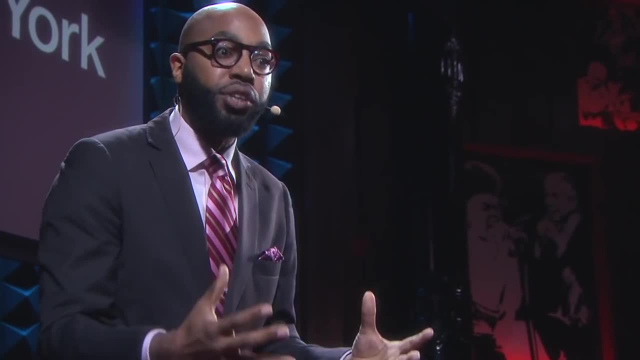 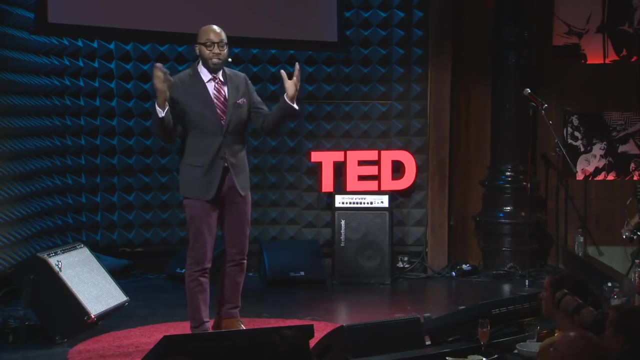 And those things are the skills that we need for the most engaging teachers. So why does teacher education only give you theory and theory and tell you about standards and tell you about all these things that have nothing to do with the basic skills, that magic that you? 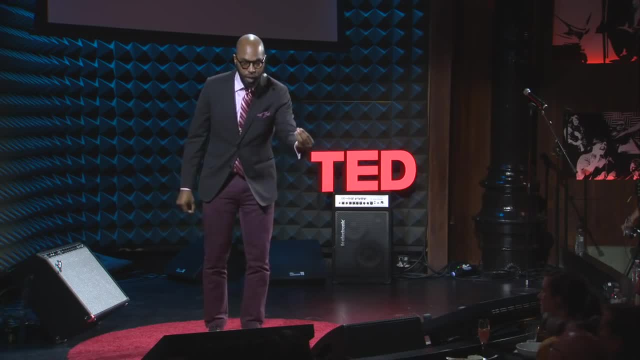 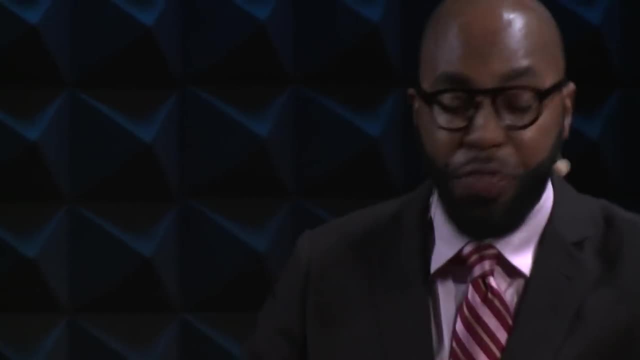 need to engage an audience, to engage a student. So I make the argument that we reframe teacher education, That we could focus on content, and that's fine, And we can focus on theories, and that's fine. But content and theories with the absence of the magic of teaching. 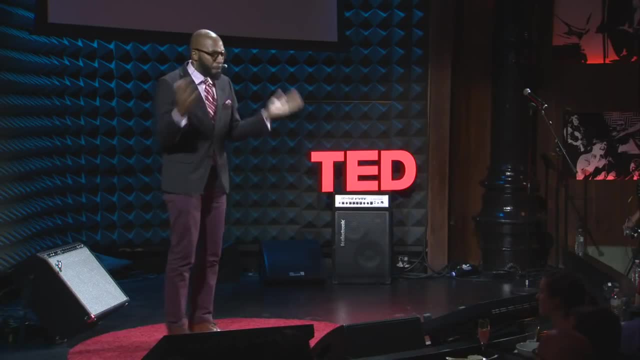 and learning means nothing. Now people oftentimes say, well, magic is just magic. You know, there are teachers who, despite all their challenges, who had those skills, get into those schools and they're able to engage an audience. And the administrator walks by and says, wow, he's. 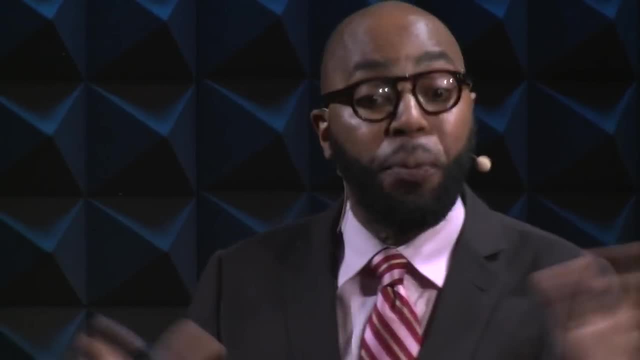 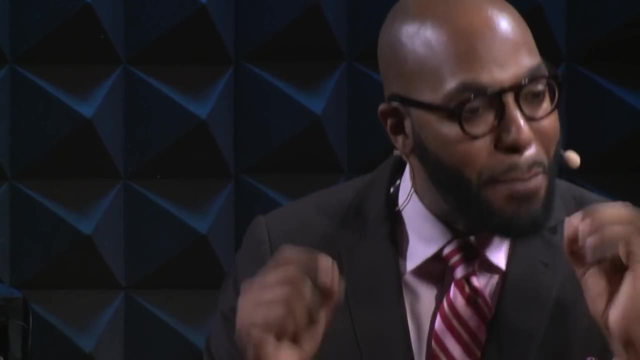 so good. I wish all my teachers could be that good. And when they try to describe what that is, they just say: he has that magic. But I'm here to tell you that magic can be taught. Magic can be taught. Magic can be taught. 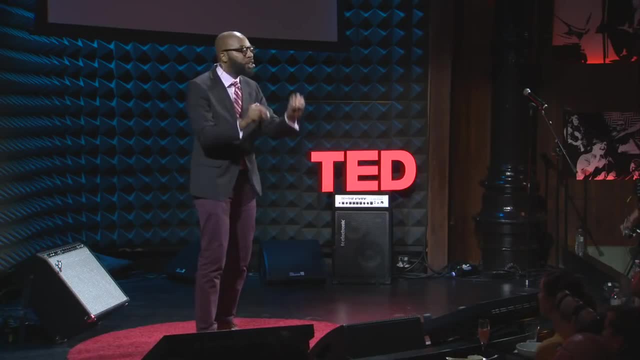 Now, how do you teach it? You teach it by allowing people to go into those spaces where the magic is happening. If you want to be an aspiring teacher in urban education, you've got to leave the confines of that university and go into the hood.